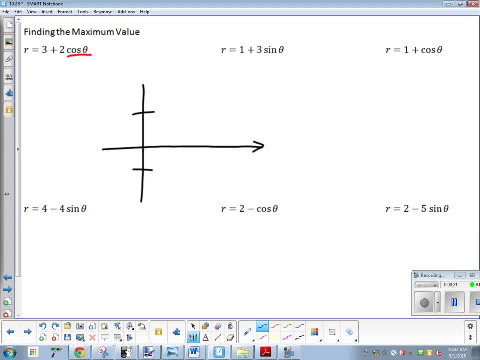 Go back and think about a cosine graph. Remember a cosine graph? Where do we start? How high do we start? if it's just cosine One, You would start at the top and then we went middle bottom. How low would we go? 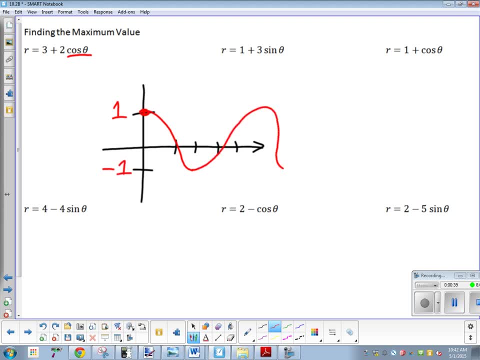 Negative one. but yeah, And then I'd go up, and then I'd go down, and then I'd go up, and then I'd go down, and then I'd go up and then I'd go down. How high does it ever get? 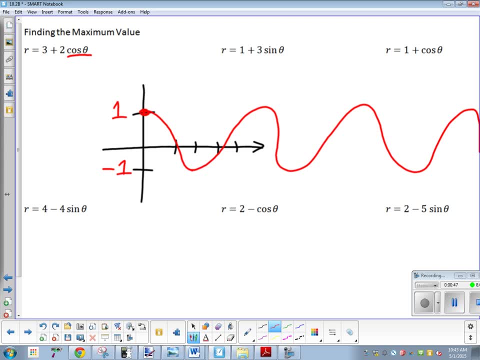 How low does it ever get? That's our only option. It goes from one to negative one, no other number. So basically for that cosine right there, I can plug in any number I want, between one And negative one, to try to make that number as big as possible, okay. 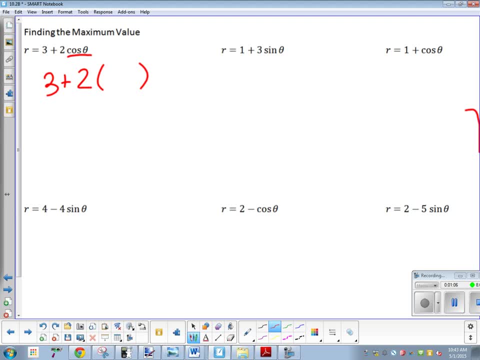 It's your only choices you're ever going to use is either one or negative one. Technically, you could use ones in the middle. You're not going to. It's not going to make it big. okay, What number would you want to plug in there to make this as big as possible? 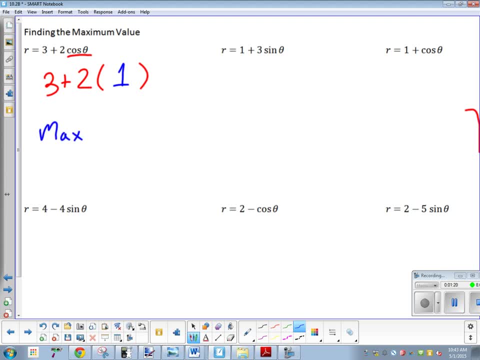 One. okay, You're going to have a maximum value. then when I plug in one, How big is that number going to be? Five? Three plus two times one gets you five. That's my max. That's as big as it gets. Then I need to figure out where. 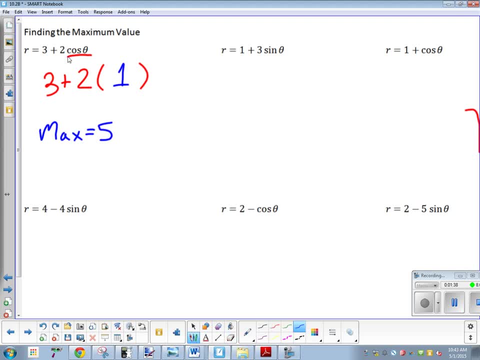 what the mess did I just make At there we go, Get my Twitter skills up. What value can I do that? Well, I need to figure out: when is cosine get me one? That's what I'm looking for. I need to look at my unit circle and decide where on my unit circle. 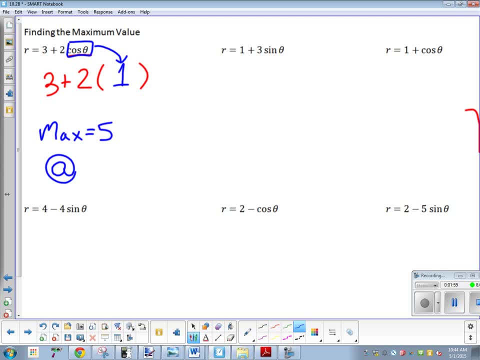 is cosine one, because that's when it's going to be the biggest. So you're looking at the full ordered pair. When is x one or cosine one Not tangent? I want cosine. So what am I looking for for cosine The x and I want to know when the x value is one. Where does that occur? 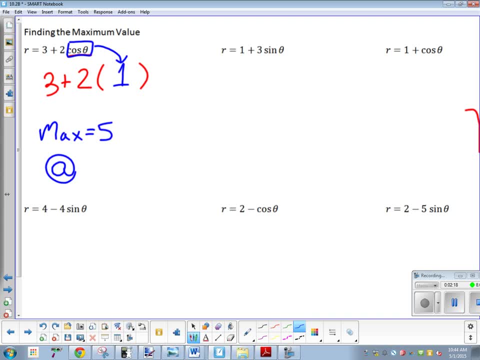 Zero. There's my x value right there. At zero degrees my x value is one, So my maximum is five. one at 0 degrees. OK, let's go to the next one. r equals 1 plus 3 sine theta. 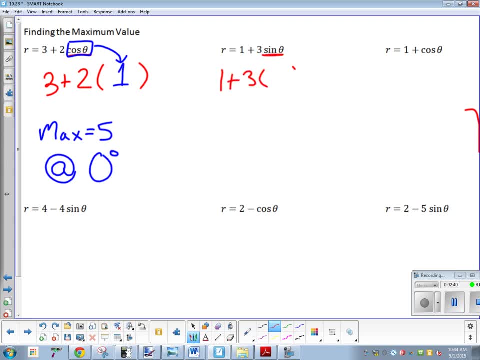 So I'm trying to figure out. what can I plug in for that? What can I plug in for sine theta that makes this number the biggest? Remember it goes from 1 to negative 1.. What number will make it the biggest 1.? 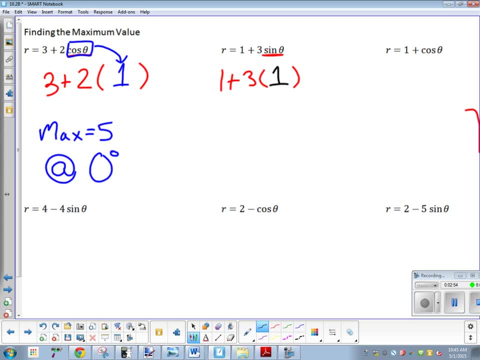 1 plus 3 times 1.. So my maximum value here is going to be 4.. That's as big as it can get. My maximum value is going to be 4.. I now need to figure out when can that happen? 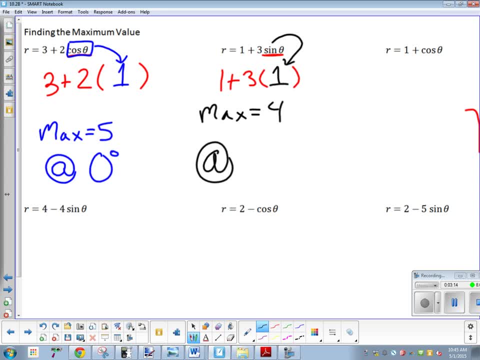 Well, that happens when my sine value gets me 1.. So I'm going to go to my unit circle again. Now I'm looking for: when does my sine value get me 1?? So what am I looking for? again, if I'm looking for sine, 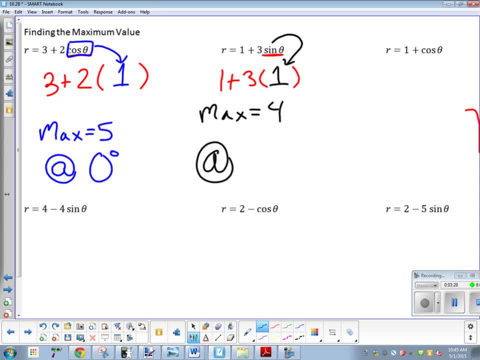 y. I'm looking for my y value up here. When is my y value going to be 1?? Right there at the top, At 1, when my y is 1, you're at 90 degrees. Your answers for these questions are always. 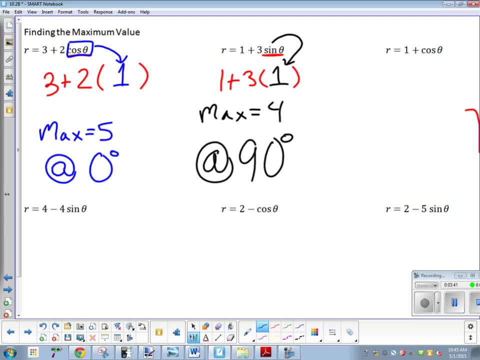 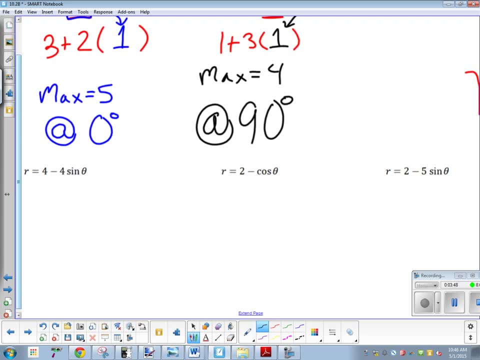 going to be either 0,, 90,, 180, or 270.. Those are your only options here. It's going to be one of the outside the straight lines. Let's skip down to this bottom one real quick. It's going to be 4 minus 4 times something. 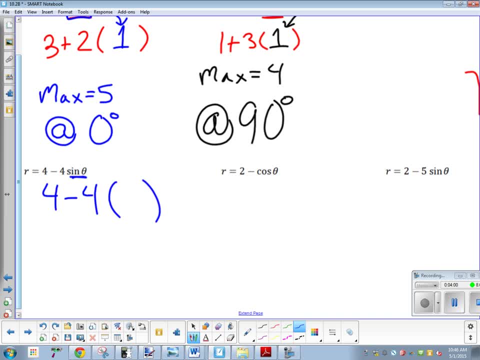 I want to plug something in for sine: theta, to make this as big as possible. What do I want to plug in for sine? Do I want to make it 1 or negative? 1? Negative, 1.. Why negative? here The minus sign. 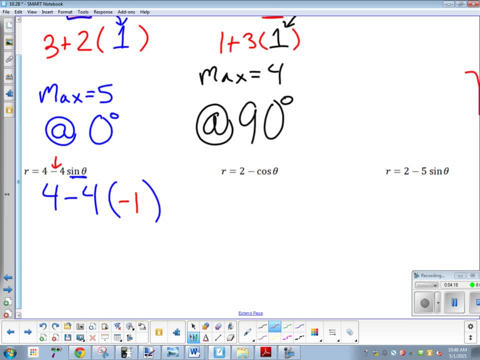 I'm going to multiply by a negative, so I want to change it to be positive, because negative 1 times negative 4 gets me positive. My max is going to be 8, and it's going to occur when sine gets me negative 1.. 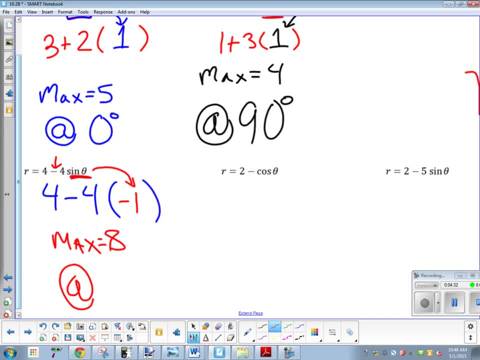 So I need to look at my unit circle and decide when is sine, when is my y value going to get me negative? 1. That's at 270 degrees.